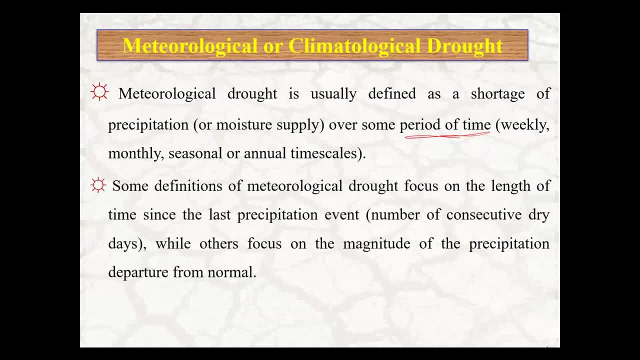 timescale, So it depends to the time. I mean that And some definitions of metallurgical drought focuses on the length of time since the last precipitation event, And you know when we say number of consecutive dry days, while other focuses on the magnitude of the. 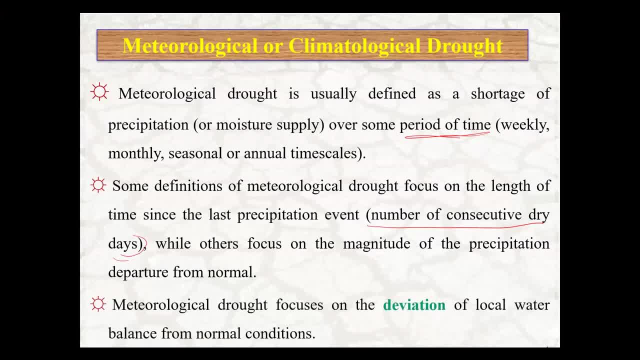 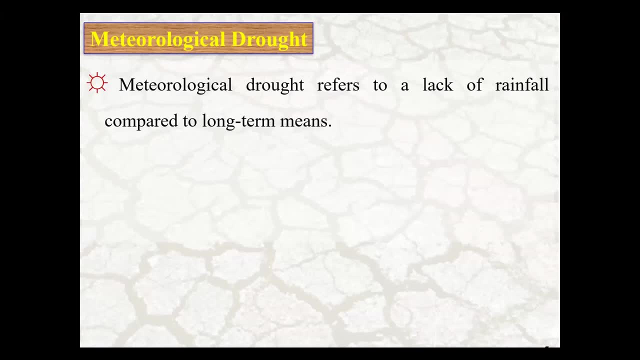 precipitation departure And also metallurgical drought focuses on the deviation of local water balance from normal conditions. There are also another definition, such as: a metallurgical drought refers to a lack of rainfall compared to long-term means And also it can be defined as period. 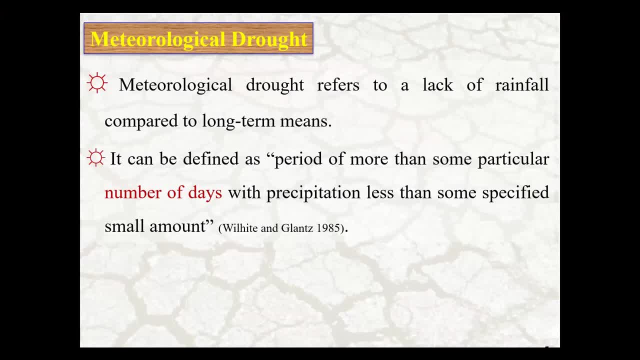 of more than some particular number of days with precipitation less than some specified small amount. And you know, just like there are numerous definitions of metallurgical drought, there are also numerous metallurgical drought indices. I will discuss more about them And, if you 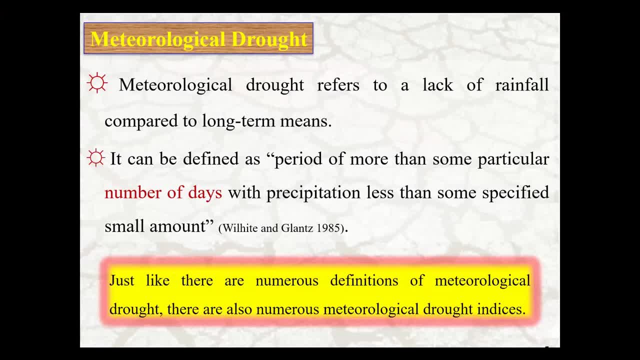 want to say that what is the cause of metallurgical drought? it's a result of a complex interplay between natural precipitation deficiencies on varying time and space scales and can be exacerbated by human water quality. And you know there are also numerous definitions. 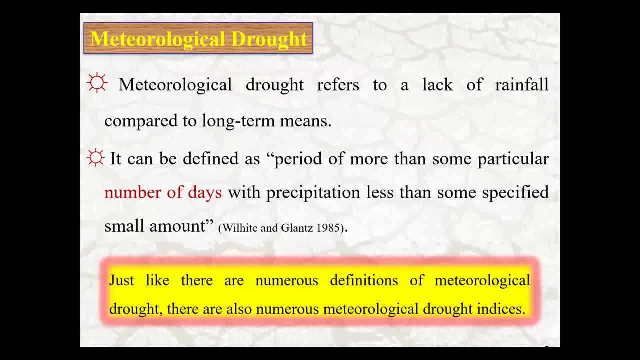 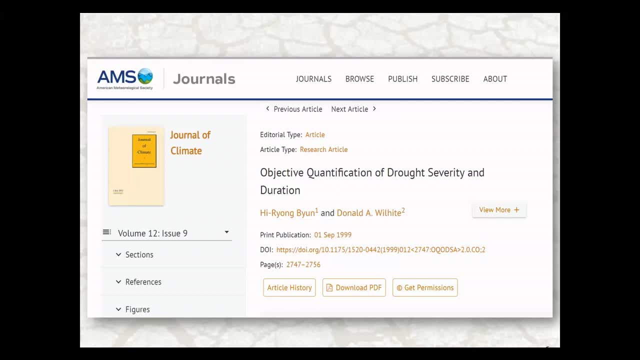 of metallurgical drought And you know, just like there are numerous definitions of metallurgical drought, And you know there are many definitions of metallurgical drought, And you know there are many definitions of metallurgical drought And, as I said, metallurgical drought it is. 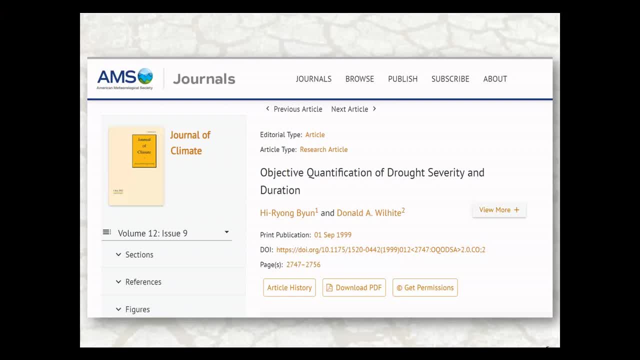 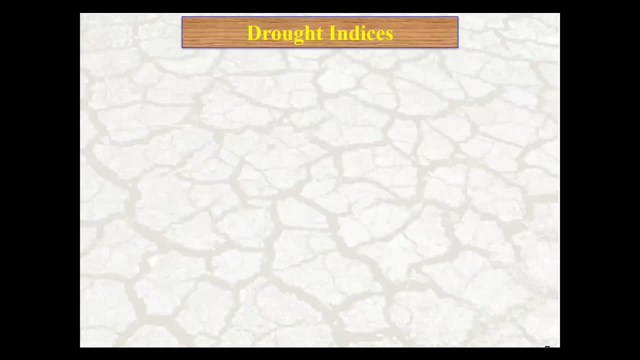 very easy to narrow down the range of rating. We need to narrow down to the rebel case in which it happens, using the spannified permeability of well-assistedisphere dumps or solid at different distances. And you know, it's very interesting that I am making examples so that people can understand more about this more precisely respected at the level of numeric imaging pitfalls. It's interesting that there's a lot of history on Skyže and other states that tell us damage is actually found however, well, whatever. And you know when you create anariamente, piezo, tore wells and moving as new measures of. 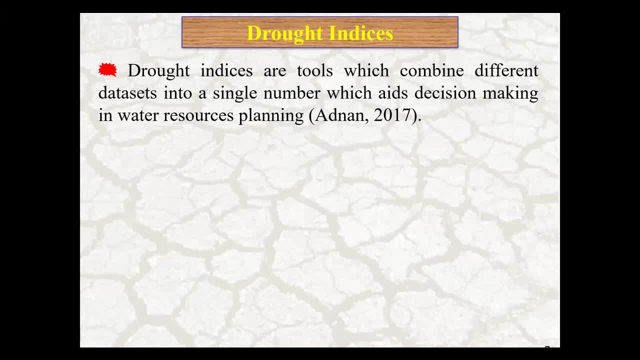 You know these are tools which combines different data set into a single number which aids decision making in water resources planning. And you know, we know that I mean there are different other concepts, for most rod indices are based on metallurgical or hydrological variables. and you know, recognition and beside 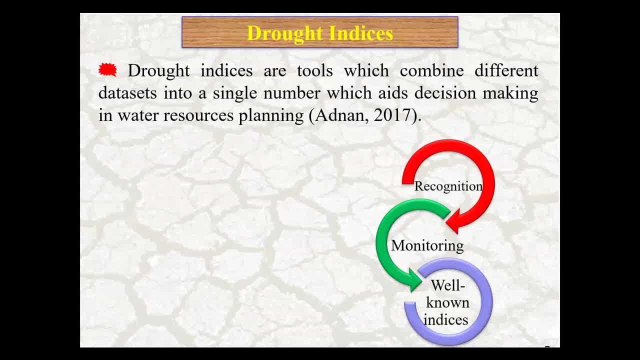 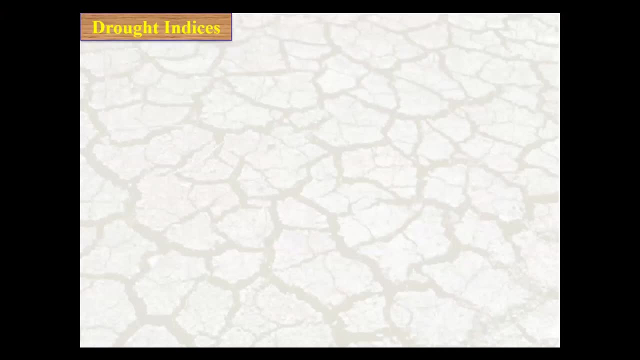 monitoring. with I mean that well-known indices are considered the first step in drought management. So we should consider this topic here for management drought and monitoring drought. So we have another things. we should know that, as I told you, most of the drought indices 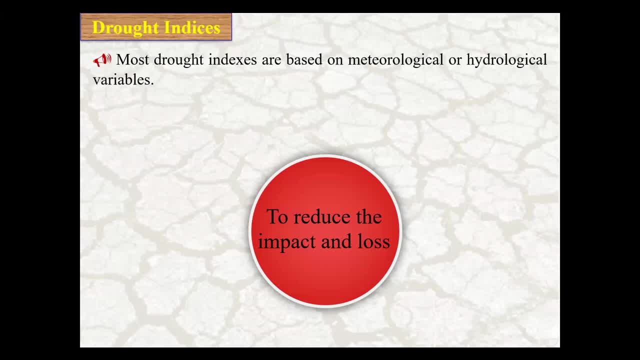 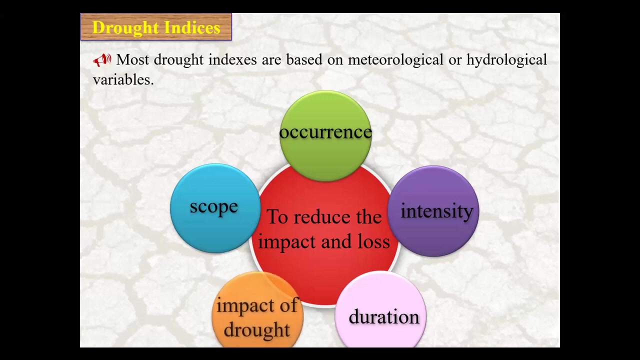 are based on hydrological variables and metallurgical variables. To reduce the impact of hydrological variables and metallurgical variables, we should consider the impact and loss of drought caused by drought. I mean that as necessary to obtain information, different information, on the occurrence and scope, intensity, duration and impact of drought. 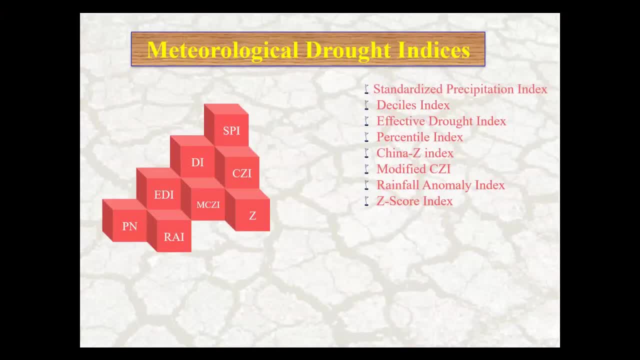 in a real time. And these are some components related to this one, You know, metallurgical drought indices. I categorize them in several, three different concepts. First of all, rain-based drought indices: eight ones such as SPI, Standard Precipitation. 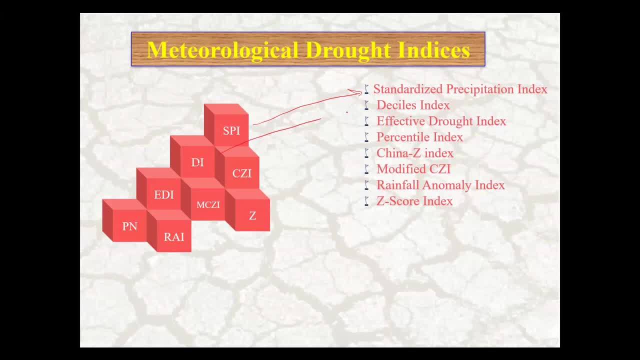 Index and, for example, DI Index, Effective Drought Index and the rest. as you can see here, these eight indices are focused on just on the rainfall as input data And another two others metallurgical. there are RDI and SPI beside precipitation. they 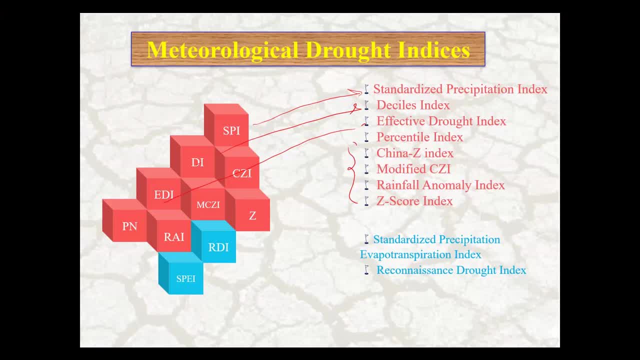 need evaporation, They need evapotranspiration data and we should consider evapotranspiration beside precipitation, KBDI and PDSI, two other elements that we consider other things such as maximum temperature and temperature data beside precipitation data. 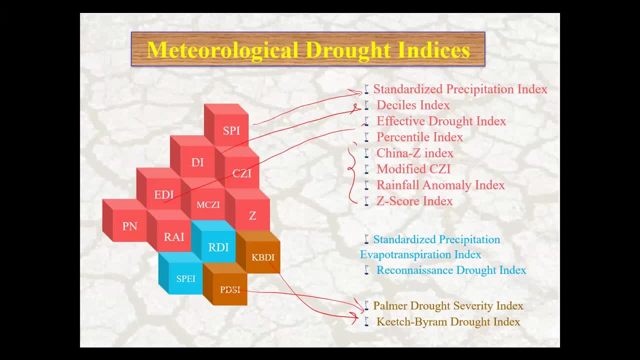 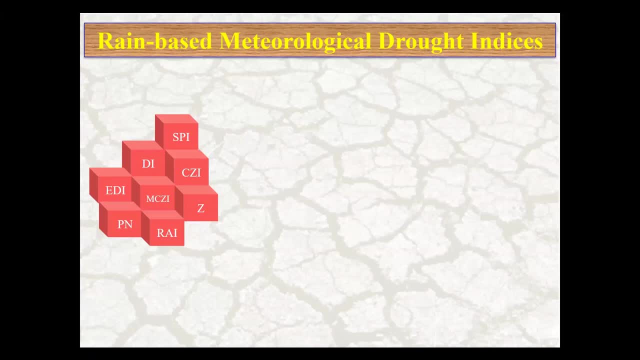 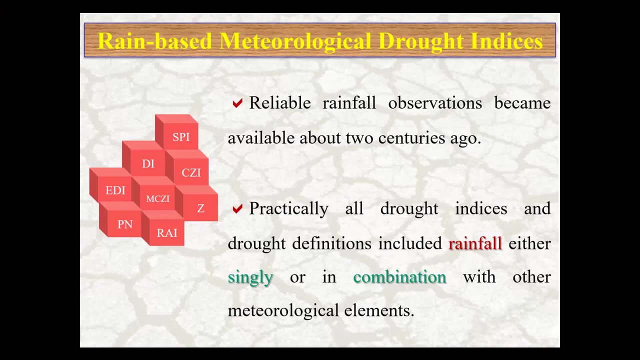 We will discuss more about these kinds of drought in the next series of video. You know, for rain-based metallurgical drought indices. we should consider that. I mean that, as you know, common to all types of drought is the fact that they originate from. 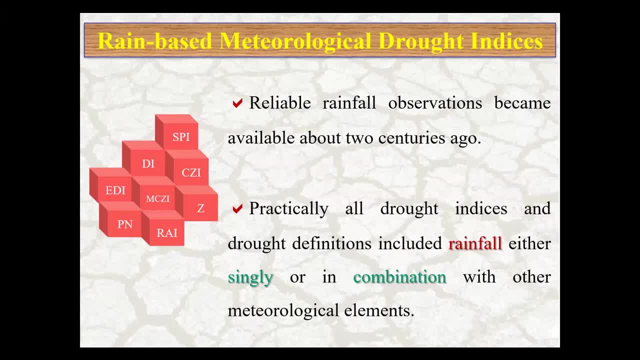 a deficiency of precipitation that results in water shortage for some activity or for some group, And fortunately rainfall is an accurate and more commonly available element of a long period of record. So practically all drought indices and drought definitions included a rainfall, either singly, 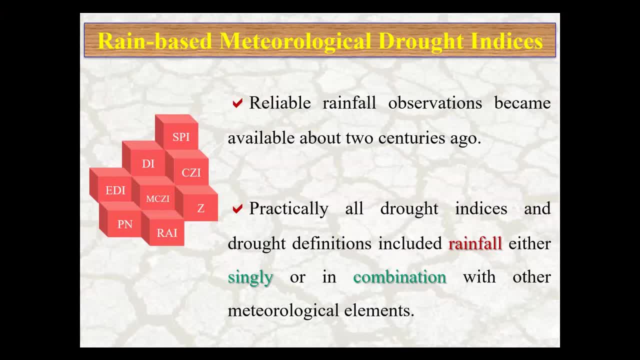 or incompatibly, And in this case it's a combination with other metallurgical elements. So we have long period of data for reliable rainfall observation become available about two centuries ago, and we can use the gridded data set, and I mean the different kinds. 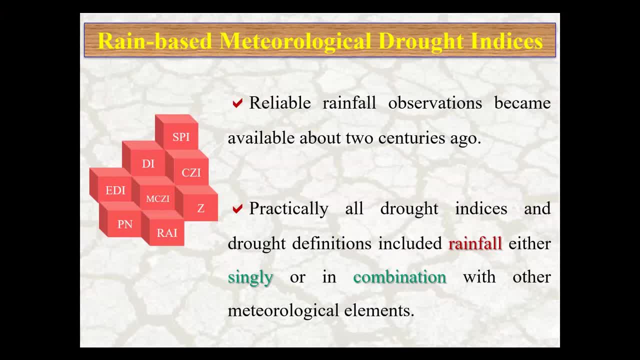 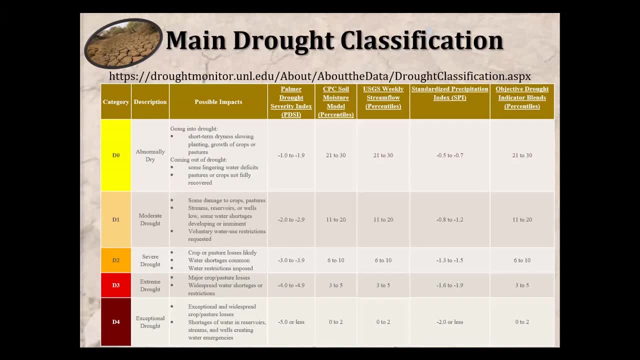 of data for rainfall data set or remote sensing data. So it's really important to know that And other things. in the last I mean the slide, The main drought classification. I will discuss it more in. you can find this table in this. 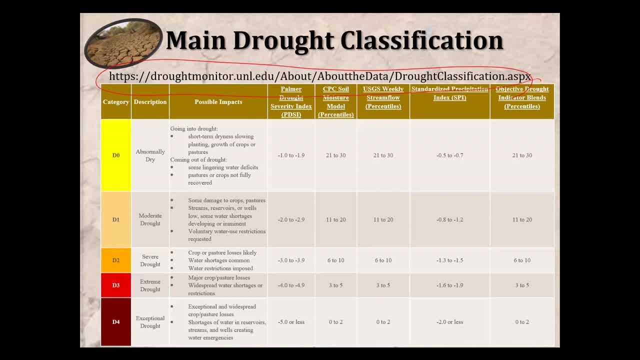 website And we have different category as a drought classification: D0, it refers to abnormal, normally dry, D1 denotes moderate drought, D2 is severe drought, D3 is extreme drought and D4, exceptional drought, And we have different indices with different classifications. 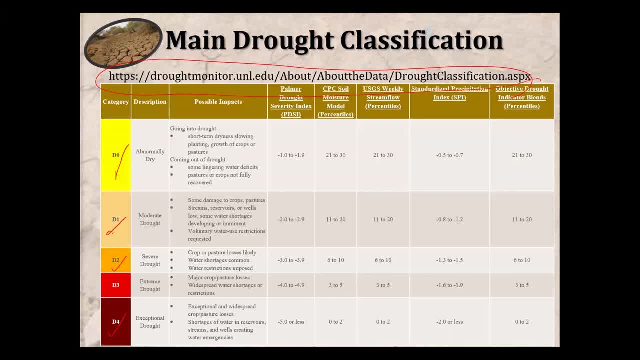 And we have different data sets And we have different classifications. but we will discuss more in next videos And you know we have different descriptions and different possible impacts. You know when we say about categorized, In next video we will focus on rain-based drought indices. 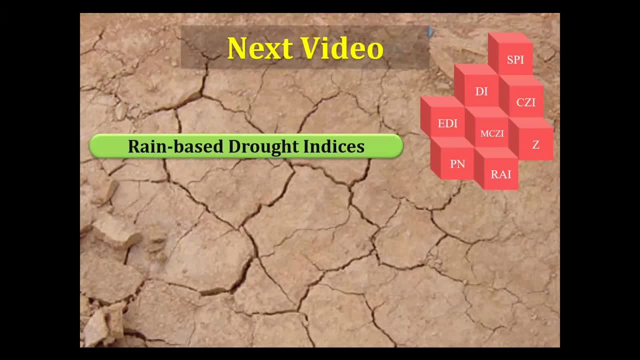 I will try to show the equations- characterization of drought indices, ecological drought indices- And we will focus on different limitations of drought indexes. I mentioned humidity. It will be a different kind, And so I have added data it's and I am this kind. 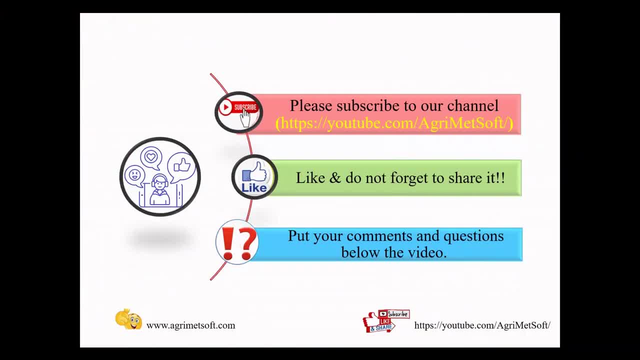 that metallurgical rain bestowal devices. okay, and now this video is finished and please subscribe to our channel. please hit the thumbs up button and don't forget to subscribe our channel. put your comments and questions below the video. would be helpful for me to know that. what are your? 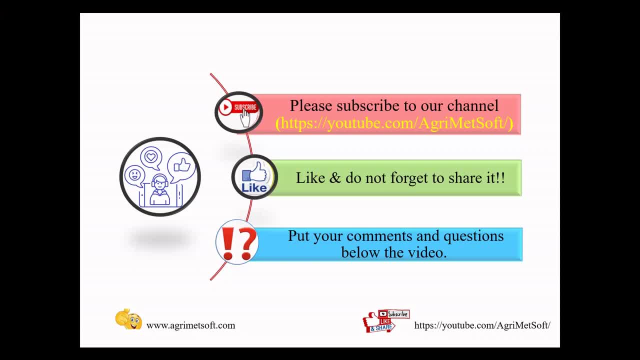 demand in this video and i hope, uh, i can see you in next video. have a good time, bye.